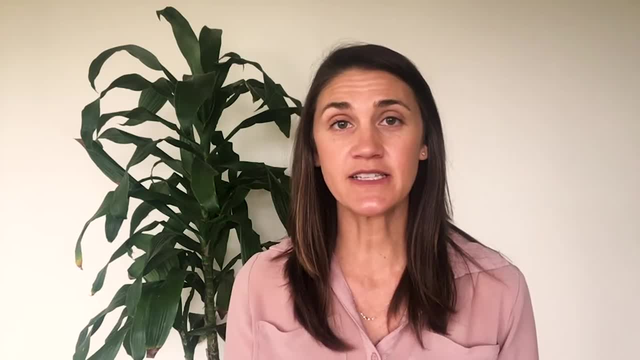 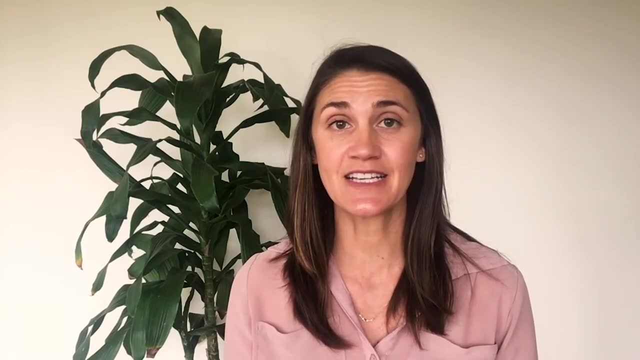 and adult life. Scientific evidence increasingly suggests that eating a low quality diet in the first thousand days raises the risk for chronic diseases such as obesity, high blood pressure and diabetes. However, many children are not eating enough high quality foods or getting enough of the nutrients they need for optimal growth and development By focusing 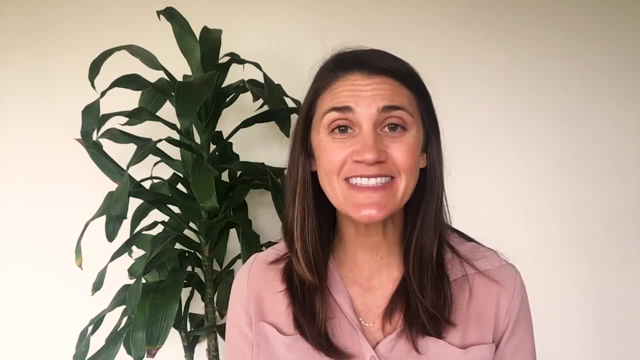 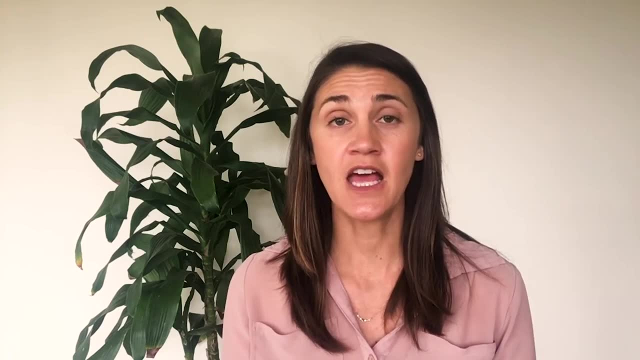 on whole, minimally processed foods such as fruits, vegetables, dairy foods and whole grains as the foundation for healthy eating patterns. children are better supported to consume the nutrients they need for optimal growth and development, reduced risk of chronic disease and better overall health. 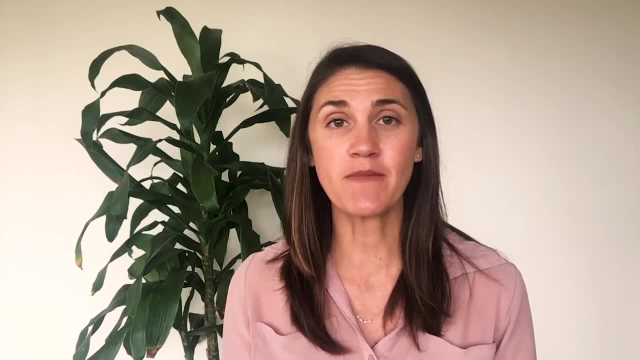 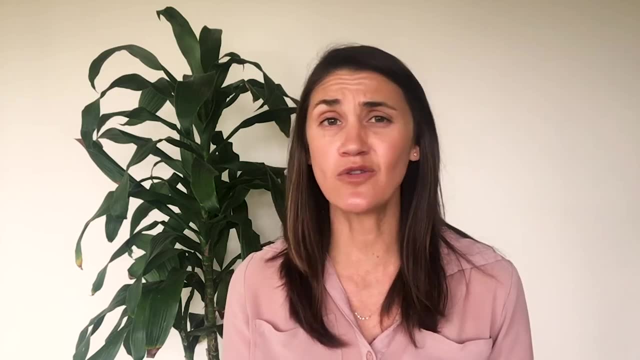 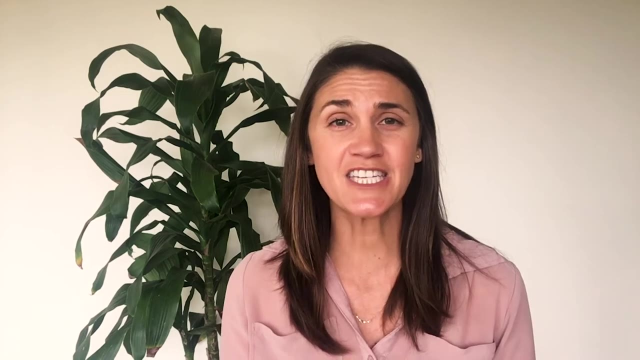 Over the past few decades, the first half of the world has seen a significant increase in the number of children who have access to healthy foods and those who do not. This results in a decline in overall diet quality for many children and families, a challenge that is hard to overcome. In fact, evidence shows that 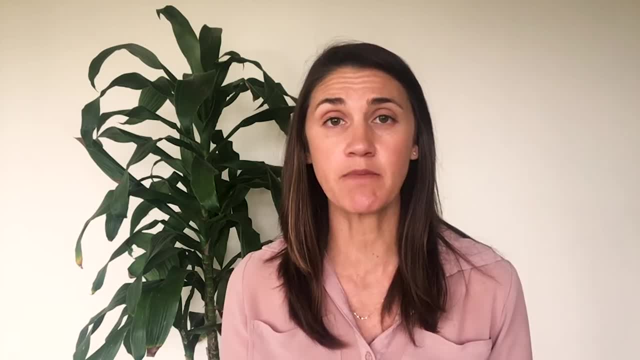 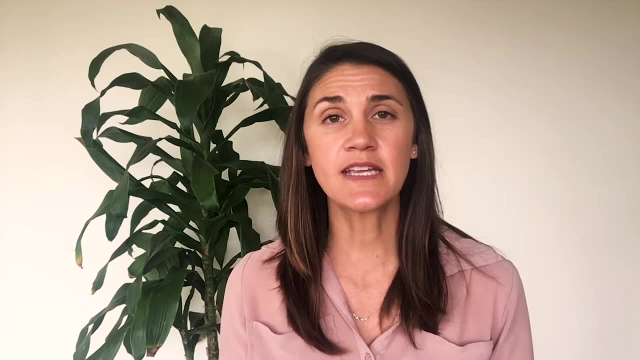 many complex factors influence food choices and eating patterns, including availability, access and affordability of healthy foods. This can even be seen as a significant increase in the number of foods or drugs- and, of course, healthとか- that are being sold for the average amount on the market. 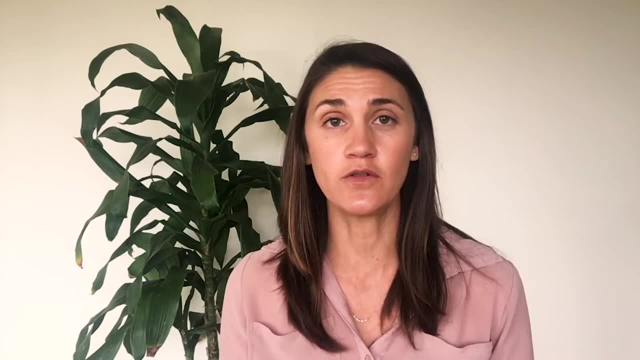 This can even be seen in the marketing and advertising of unhealthy foods and beverages directed towards children and their families. These factors, also called social determinants of health, can create barriers to making healthy food choices. Fortunately, the educational environment today continues to shift toward a more holistic view of health, expanding 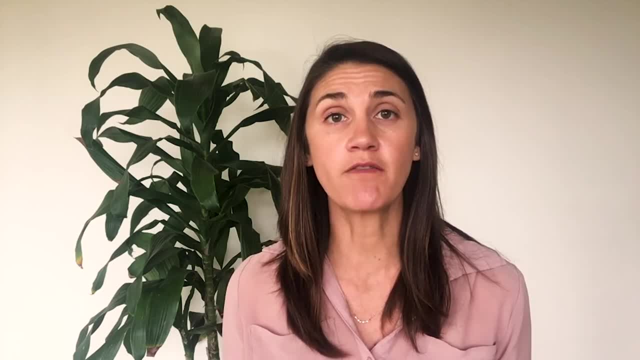 beyond traditional subjects and to also support the needs of the whole child—a dragon and a fly—in order to stay healthy and ultimately work with other children, in order to change the way that they think of health and their experiences of all of us as adults. 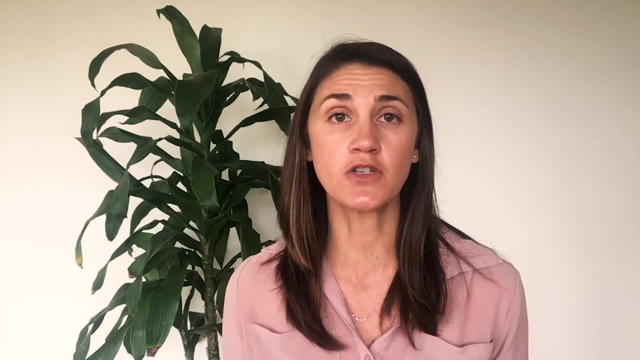 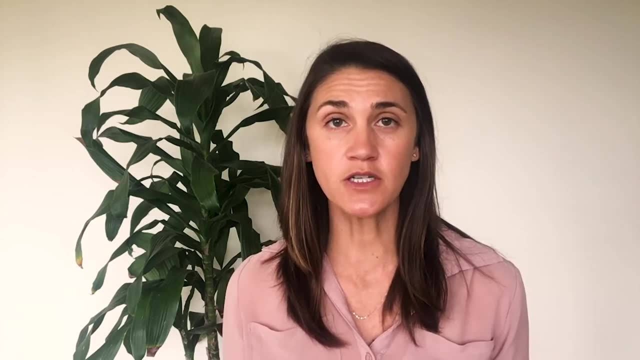 This can even be seen in the marketing and advertising of unhealthy foods and beverages. addressing their social and emotional well-being, This provides an opportunity to teach nutrition education, which it is an important tool to help children and their families understand the difference between healthful and unhealthful foods.